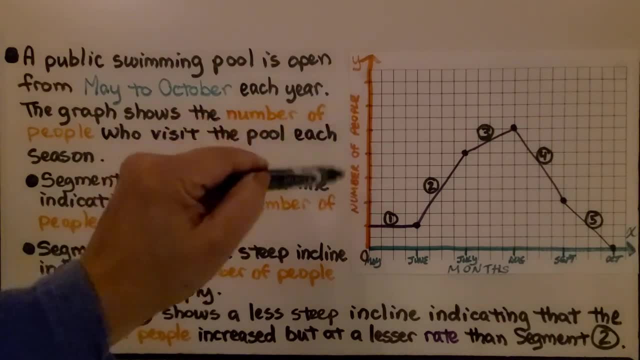 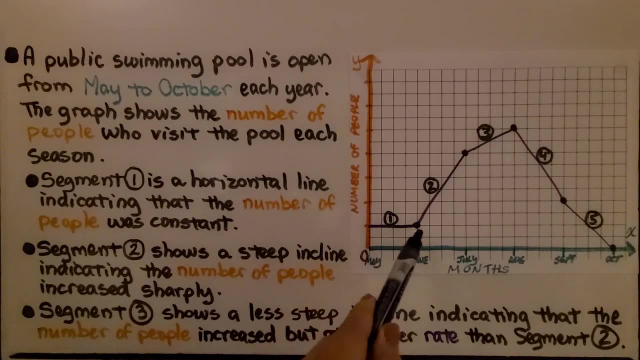 The graph shows the number of people Who visit the pool each season. Segment 1 is a horizontal line, indicating that the number of people was constant. Segment 2 shows a steep incline, indicating that the number of people increased sharply. And segment 3 shows a less steep incline. it's not as steep as 2,. 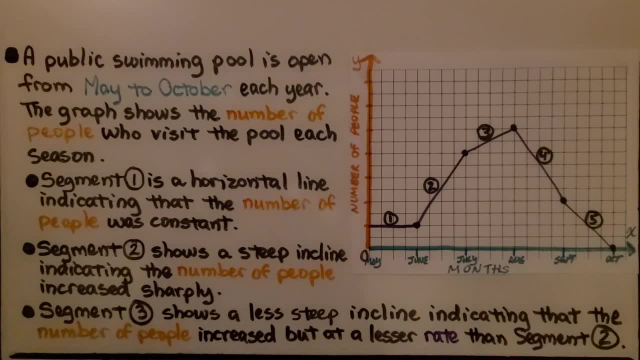 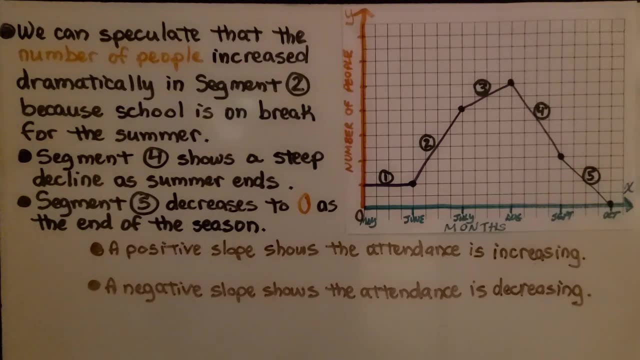 indicating that the number of people increased, but at a lesser rate than segment 2.. We can speculate that the number of people increased dramatically in segment 2 because school is on break for the summer, That's from June to July, And segment 4 shows a steep decline as it's approaching September and summer is ending. 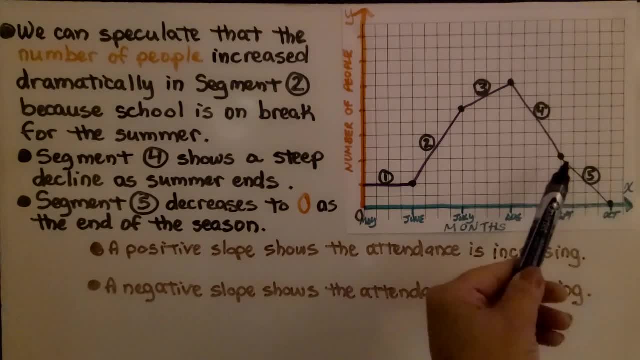 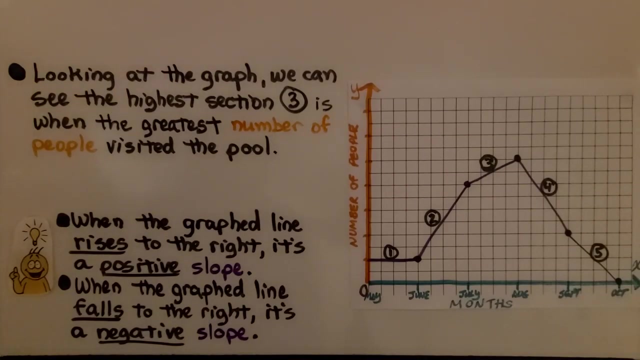 And segment 5 decreases to zero as it is the end of the season when the pool is going to close. So a positive slope shows the attendance is increasing And a negative slope shows the attendance is decreasing. Looking at the graph, we can see the highest section 3, is when the greatest number of people visited the pool. 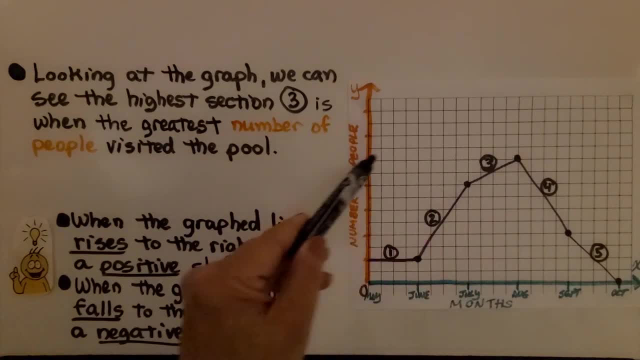 Here's the number of people and that's the highest point, And when the graph line rises to the right, it's a positive slope, And when it falls to the right it's a negative slope. So we can see the number of people are decreasing. 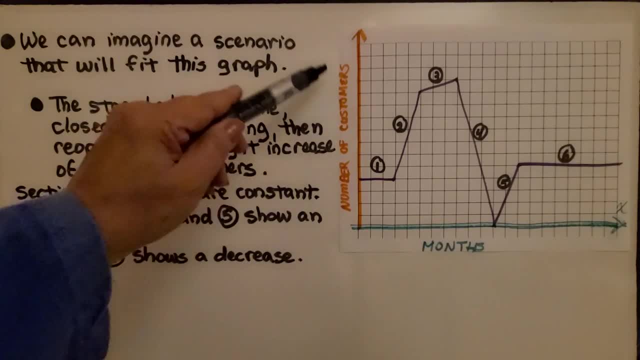 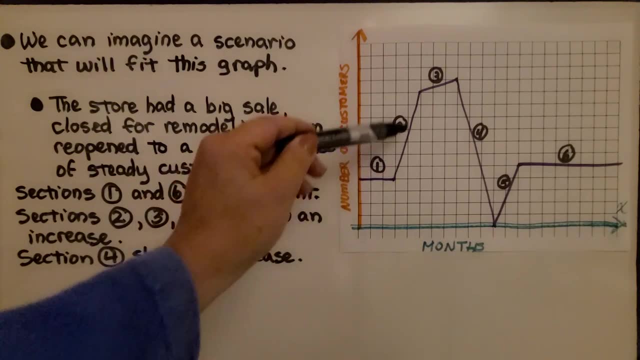 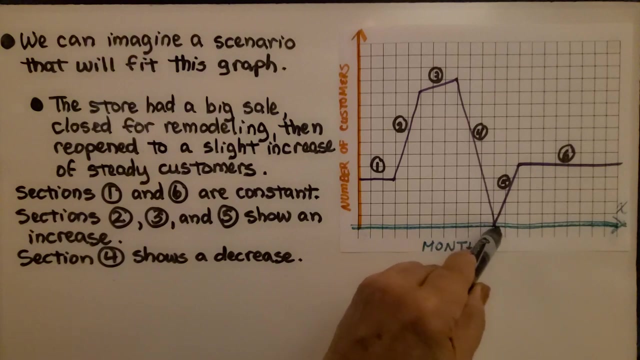 Now take a look at this graph. This is the number of customers and this is the months that the business was open. Look what happens: It goes steady, It increases, It increases slightly, Then it falls dramatically all the way down to the x-axis where y is zero. 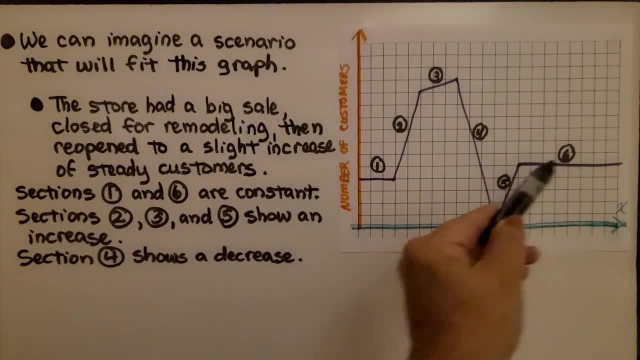 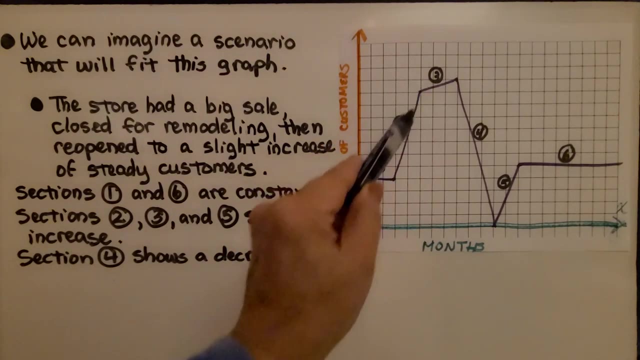 And then it goes up and then it's constant again, But look, it's higher than in the beginning. We have a constant here, but now it's raised up. So we can imagine a scenario that will fit this graph. We can think the store had a big sale, sold a lot of things and then closed for remodeling. 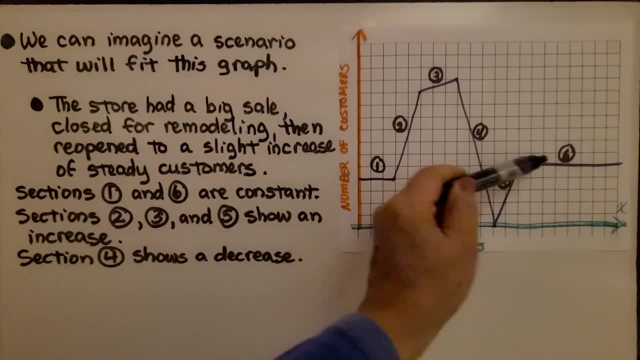 And then reopened to a slight increase of steady customers. We can see section 1 and 6 are constant And sections 2, 3, and 5 show an increase. We have an increase, an increase, and then we have another increase here.